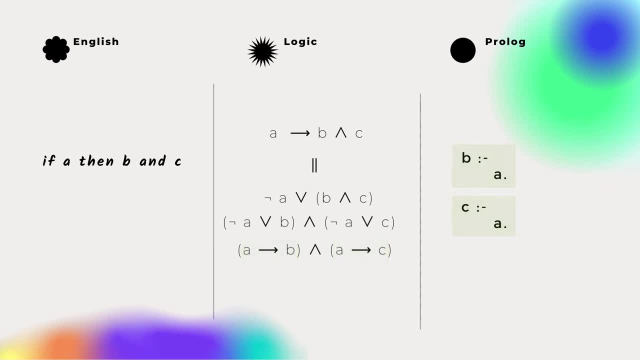 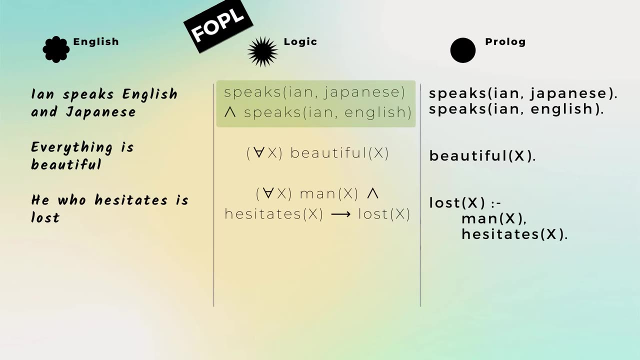 Each one of these becomes an individual prologue rule. Predicate logic follows the same pattern. Predicates that are conjoined together become individual prologue facts And for universal quantifiers, every variable in a prologue rule or fact is implicitly universally quantified. 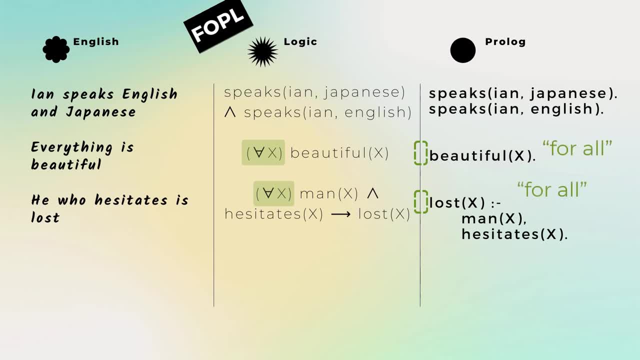 So this fact and rule mean for all x, even though it's not explicitly written. Sometimes the natural language counterparts are normal sentences, but sometimes they are sayings: Everything is beautiful, he who hesitates is lost. The bottom line gives you the most general form of a prologue rule. 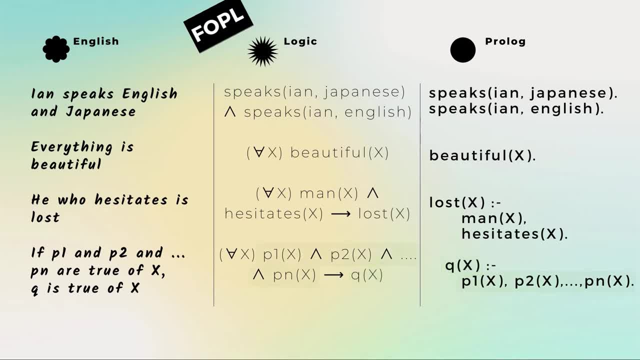 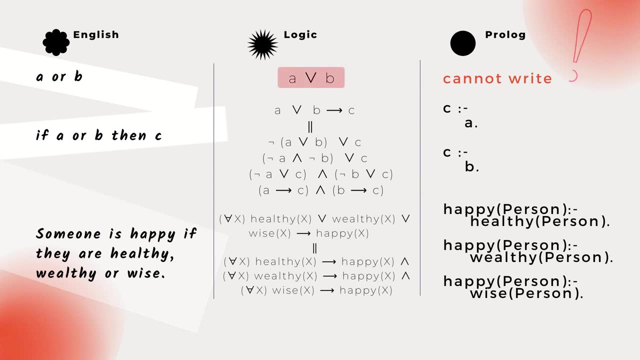 One non-negated predicate as the head and on the right any number of predicates conjoined together by commas. So dealing with, AND looks good. How about? OR In its simplest form? there is no way to directly express, just A or B. 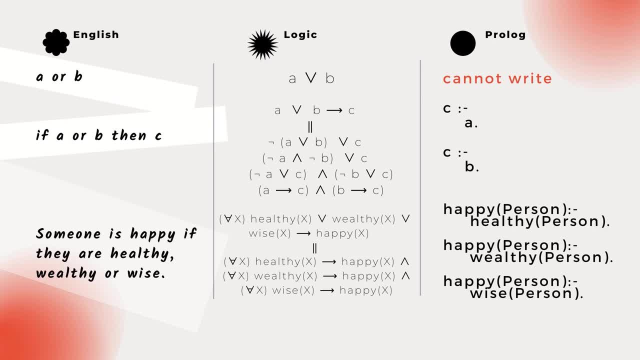 Where we can express OR is when it occurs in a sentence OR is in combination with other operators, Especially when it's on the left side of an implication. it can be rewritten into two simpler implications. Each of these translates into a prologue rule, as we've already seen. 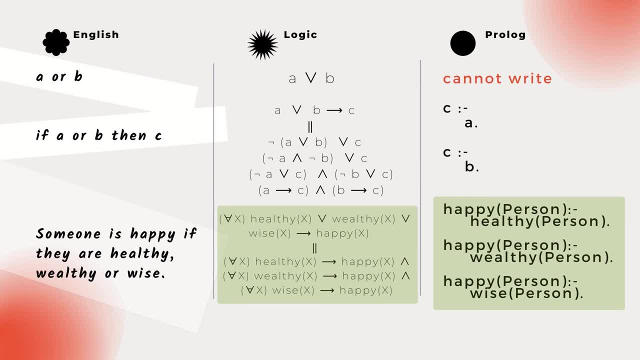 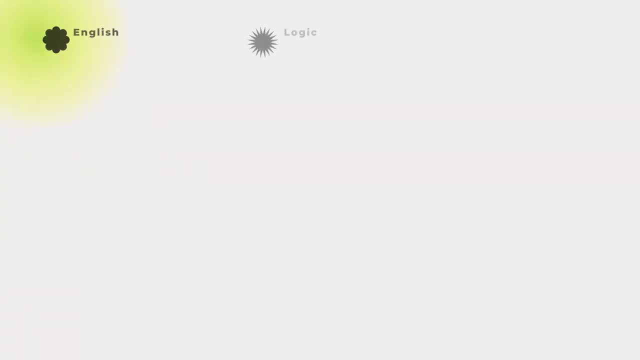 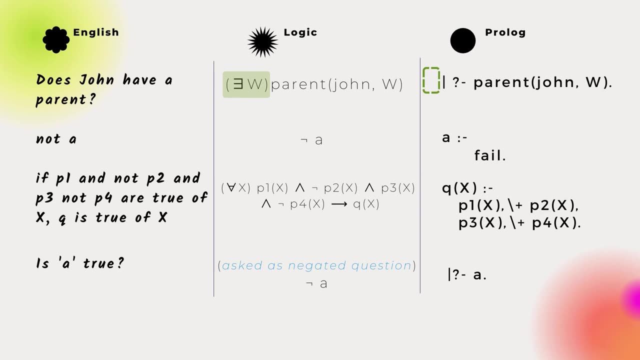 And this translation works for predicate logic. Predicate logic also has existential quantifiers. Like universal quantifiers, these are represented only implicitly in prologue. Every variable in a query is existentially quantified. Existential quantifiers are presented here with negation for a reason. 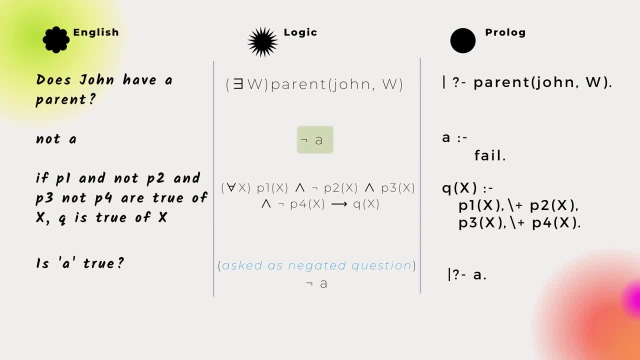 Although it's not common for individual predicates, there's a way to express negation using the impredicate FAIL, And the predicates in the body of a rule, but not the head, can be negated, So expressions like this are also OK. 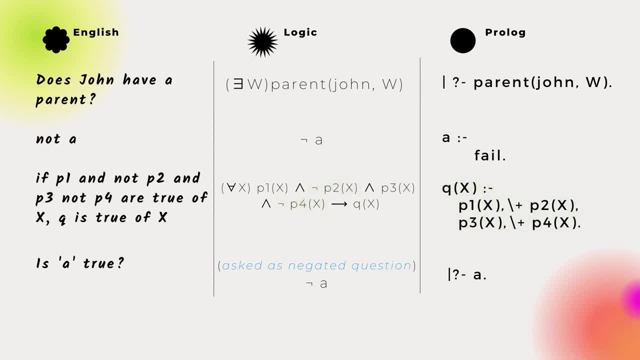 But prologue has a more natural way of interpreting negation, which is implicit, like its representation of quantifiers. A query is actually the native way of using negation, Since prologue is based on doing proof by contradiction. The easiest ways to see this are to compare resolution proofs and prologue search and. 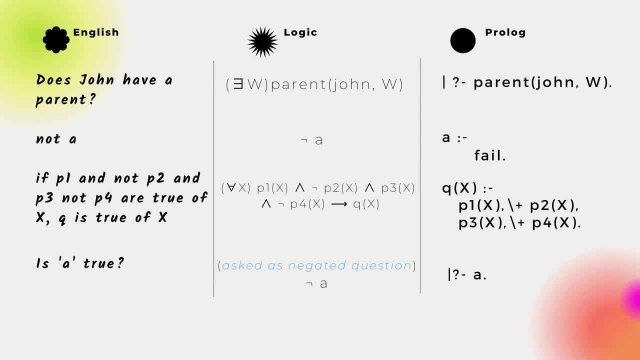 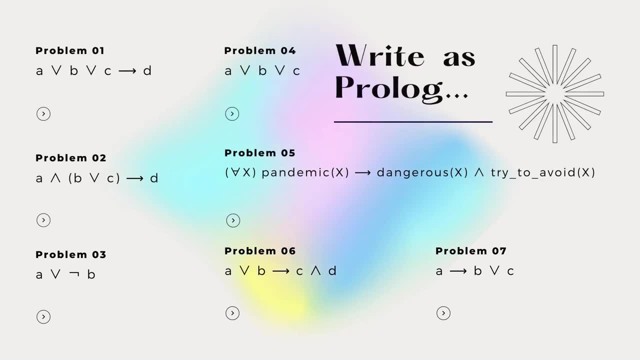 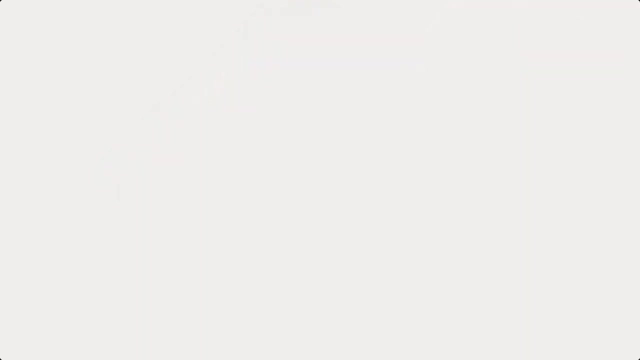 to understand the three types of horn clauses. For now, test your knowledge with these questions on logic and prologue. Thank you for watching and I'll see you in the next video. 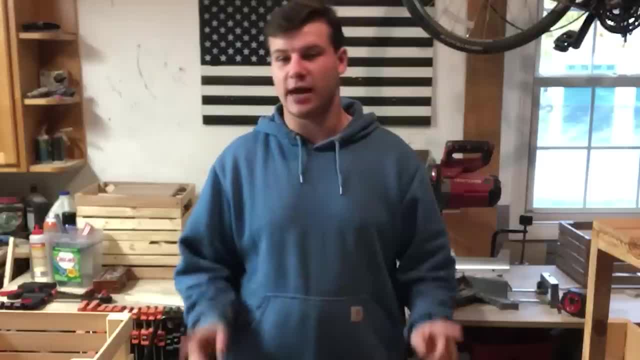 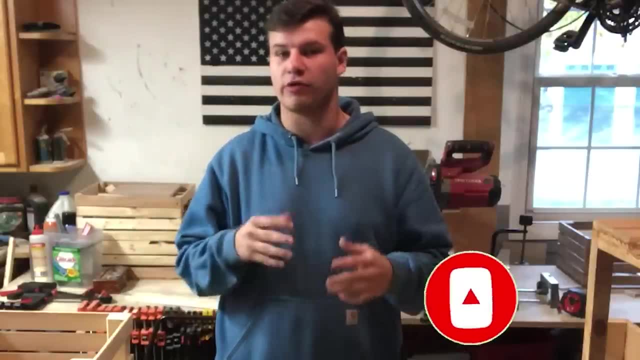 What's up guys? Welcome back to Fisher Over Tricks Woodworking. My name is Peter and today we're going to be going over 40 projects that sell 40 projects that I have made and you can make, and most of them are small projects. There are some bigger things in there, like coffee tables. 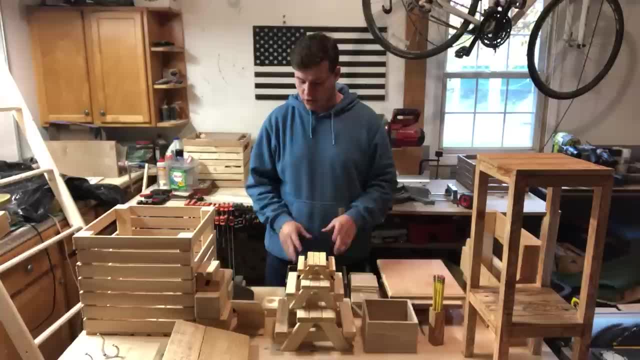 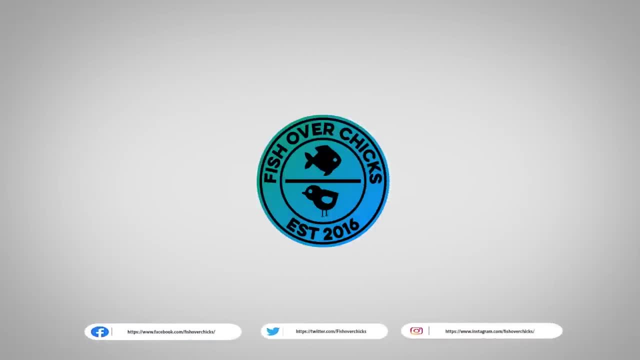 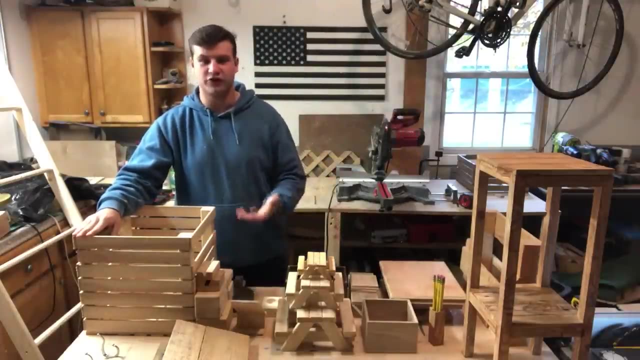 and benches, but for the most part they're smaller projects. They don't take a lot of wood and they're fairly cheap to make, So let's get into it. Number one is a. crate Crates are great because they can hold everything that you've just made. 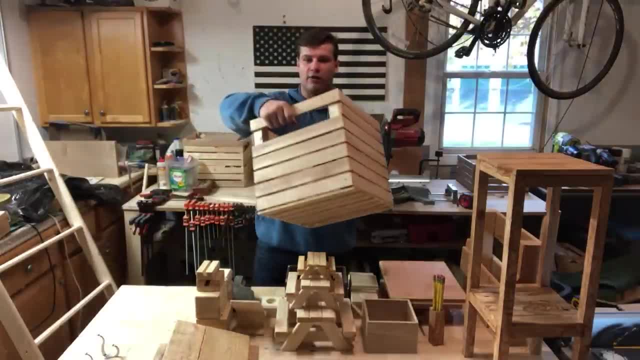 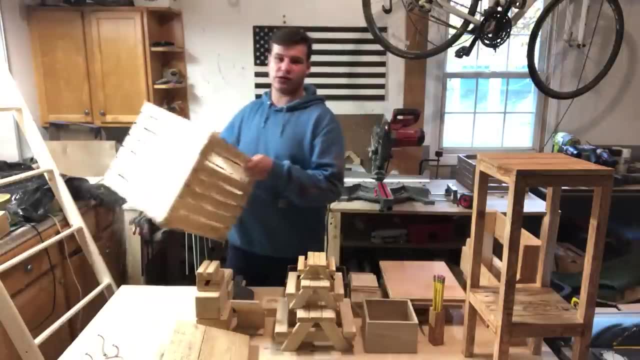 right in there. So crates are great. This one I made out of just 2x4s and I actually have a video on how to make that on my channel. I'll put it up in one of these corners there. These sell really. 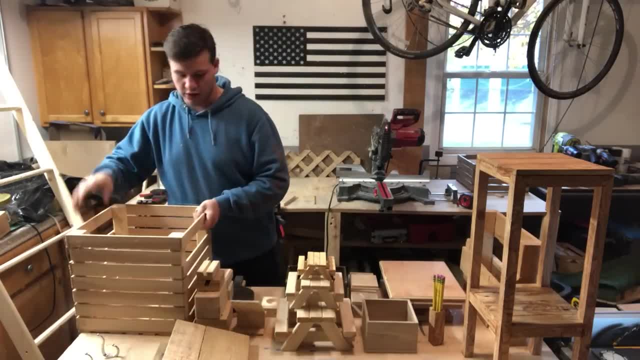 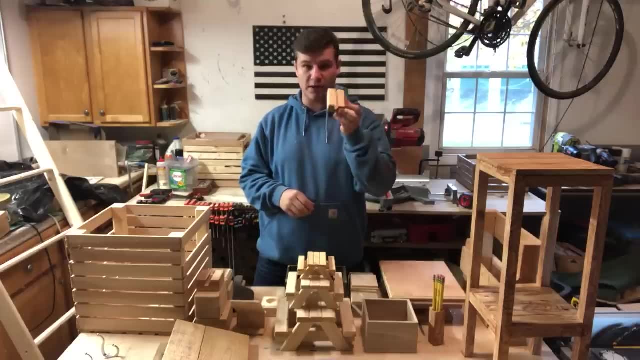 good. People love crates. They look nice. So yeah, crates. number one. Number two: business card holders. Business card holders are really good. They're really good, They're really good, They're great, because everyone needs a business card holder. It's just a little piece of cedar and 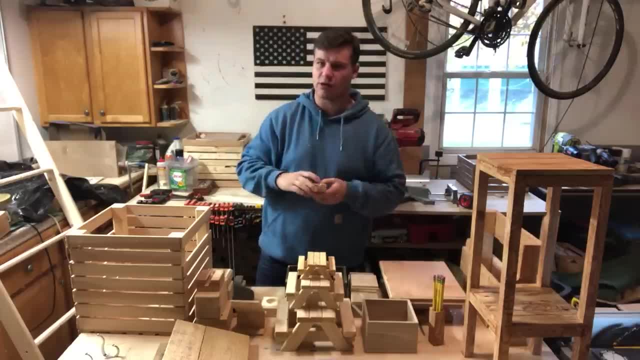 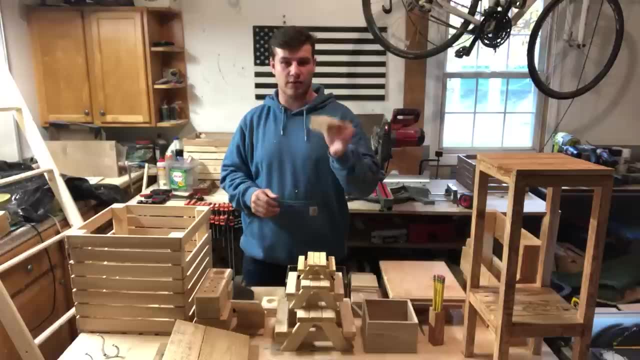 then you just cut some slits in it with a table saw at an angle. It's super easy to make. So business card holders are number two. Number three is basically the same as a business card holder, but it's a little bit bigger. It's a piece of a 2x4 and it is a phone holder. I've got five.